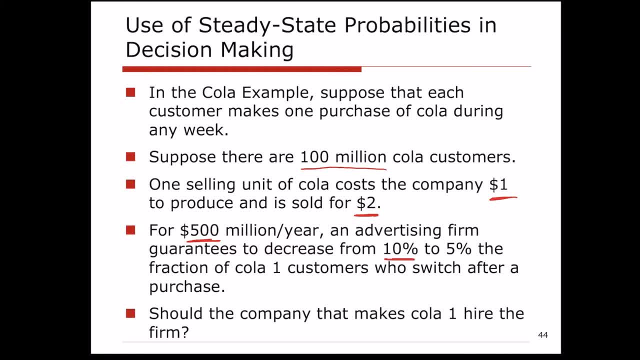 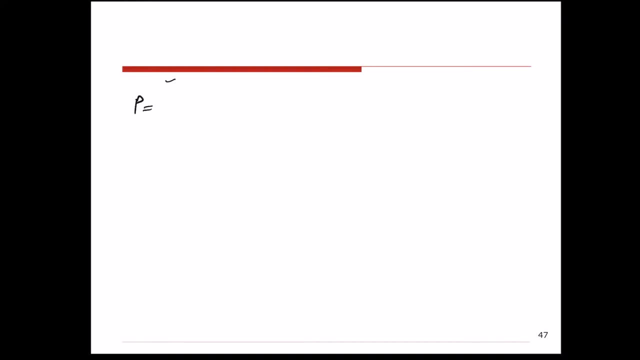 In the next purchase from 10% to 5%. So then the question is that should the company that produces cola 1 go ahead and pay for this ad or not? Let's look at the problem again. So in the previous scenario, the one is the transition probability metrics was as these metrics, And and then the steady state probabilities that we calculated was 0.67 for cola 1 and 0.33 for cola 2.. 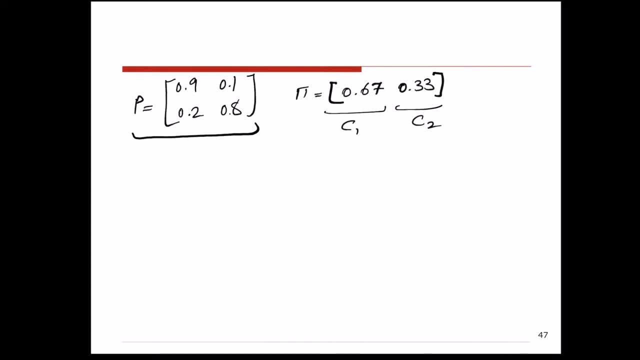 So, and as it was stated in this problem, we have $100 million customers. Okay, so what does that mean? So that means that in the steady state, when this system reaches equilibrium, if we stop the system and pick any random customer, we expect that with the chance of 67%, that person is drinking cola 1 and with the chance of 33%, that person is drinking cola 2.. 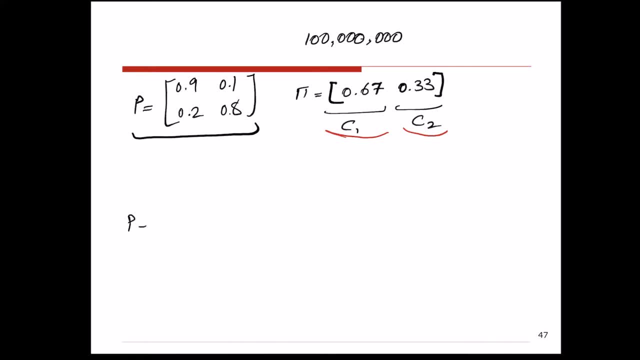 Now this company has the possibility of initiating some advertisement And this advertisement is supposed to change the percentage of people that are switching from cola 1 to cola 2 to 5%. So this advertising company is supposed to change the percentage of people who are a cola 1 drinker right now and in the next person are going to change to cola 2 to 5%. 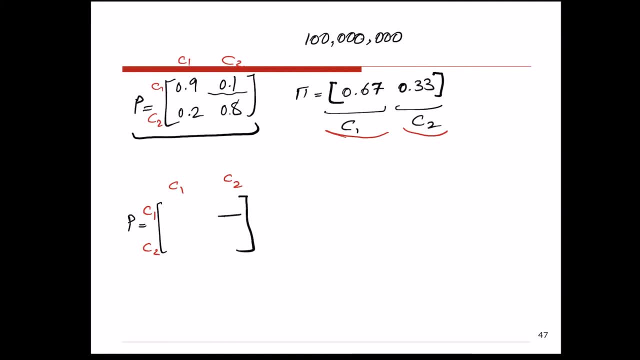 So the initial value was 10%, So it's supposed to go down to 5%. So if that happens, then the probability of a person who is a cola 1 drinker sticking to cola 1 in the next purchase is going to go up to 95%. 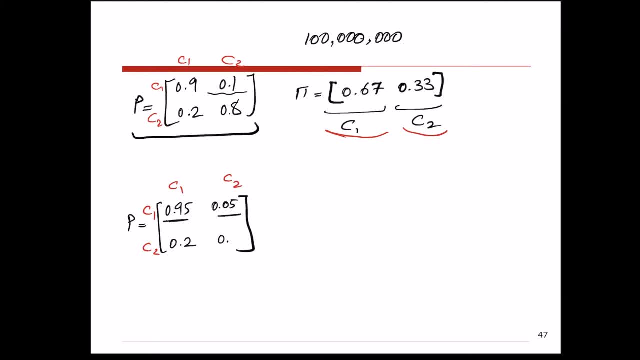 And so nothing changes with respect to cola 2.. So the question is that should this company go ahead and pay half a million dollars for this advertising and make such that they can make this change in the one step transition probabilities? So should we do that or not? 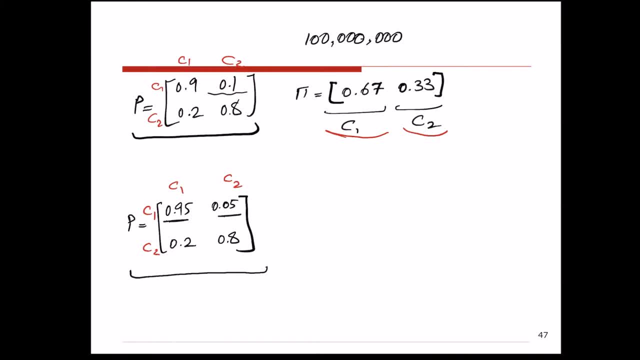 What we have to do in this system, in this scenario, to be able to answer this question is to go ahead and find the city-state probabilities under this setting to find out what is the chance that in this setup in the long run in the city-state. 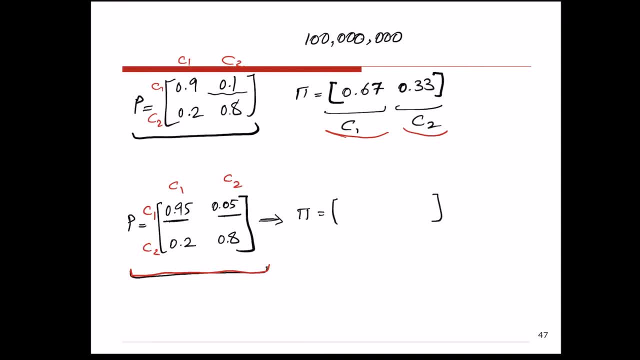 if we stop the system and we pick a person, a random person, what is the chance that the person is cola 1 drinker And what is the chance that the person is a cola 2 drinker? So basically, the values of pi 1,. 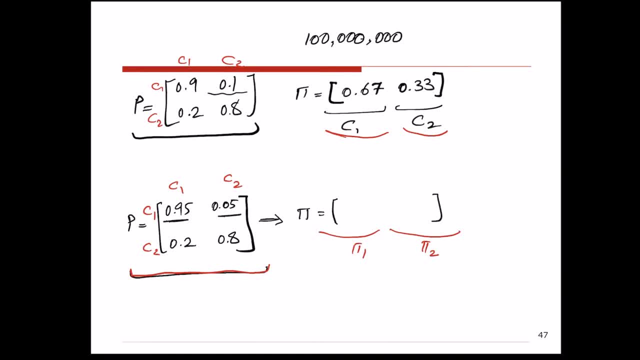 and pi 2 are going to tell us what is going to be the market share of cola 1 and cola 2.. Once we find the percentage of people that are drinking cola 1 and drinking cola 2 in the long run, we can see how the market share of cola 1 has changed by this change in the transition in the one step transition probability matrix. 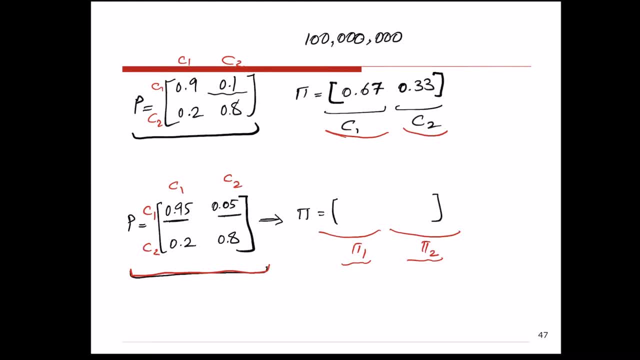 And if that change in the market share would bring enough profit to justify the half a million dollar that we have to pay for the marketing part. So let's go ahead and find pi 1 and pi 2 related to this new transition probability matrix. 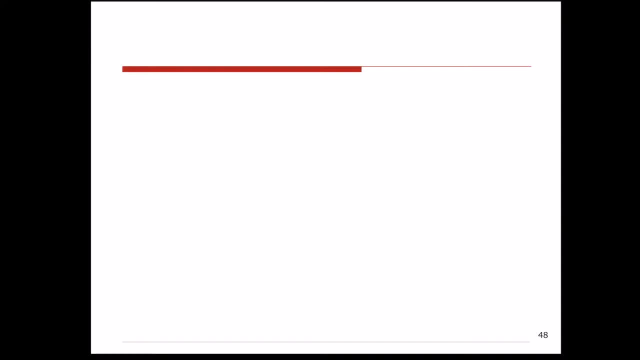 So the formula that we have to follow is: pi multiplied by 1 is the transition probability. matrix P equals to pi. So that's going to be now we can go ahead and do the matrix multiplication. So we have to multiply vector pi by the first column of matrix P. 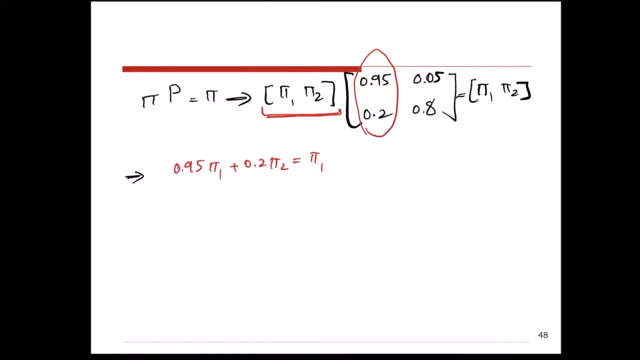 That's going to be. and similarly, we have to multiply vector pi by the second column of matrix P, And that's going to be. So here we have two unknowns, pi 1 and pi 2, and we have- we need- two independent equations to be able to find these two unknowns. but, as we stated in, 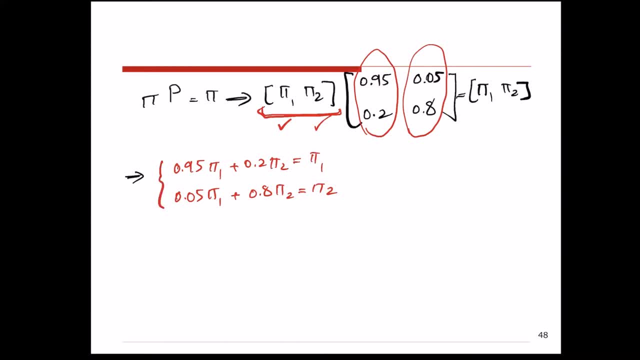 previous video when we put the equations related to pi: P equals to pi we. One of these equations is going to be dependent to the rest of the equations, so we can drop any one of these equations. It doesn't matter. We can drop any one of them and add the other equation that we know is always true for any. 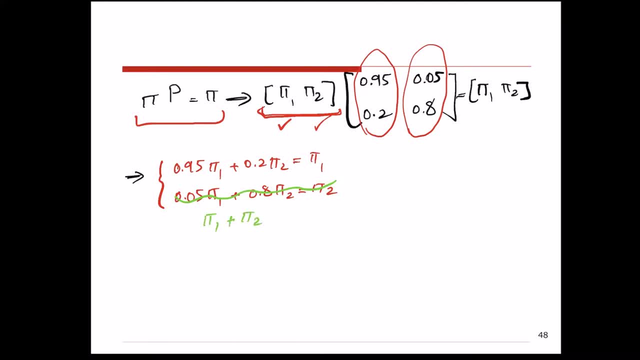 stochastic system, Pi 1 plus pi 2 equals to 1. now We have two equations, equation 1, equation 2. these two equations are independent from each other. We can solve these set of equations to find the two unknowns, pi 1 and pi 2. and if we do that, 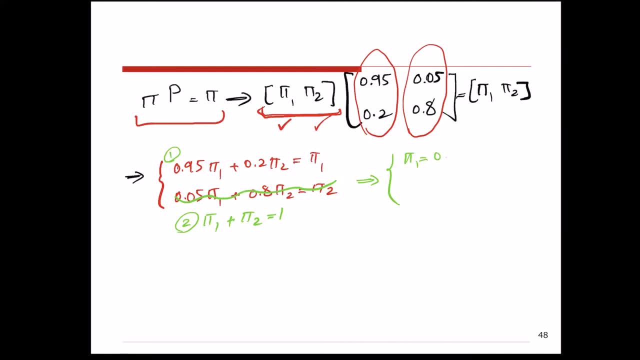 The values. the new values for pi 1 is going to be 0.8 and the new value for pi 2 is going to be 0.2. What does that mean? That means, with this new transition probability matrix that we will get if we perform the 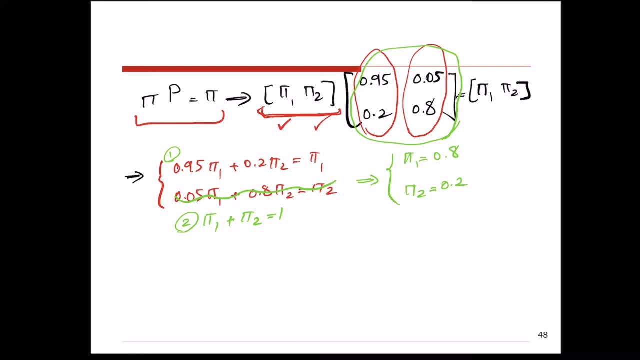 Advertisement: in the long run, when the system reaches the steady state or equilibrium, If we stop the system and pick any random person from this population, there is 80% chance that the person is drinking cola 1 and 20% chance that the person is drinking cola 2. so in other words, 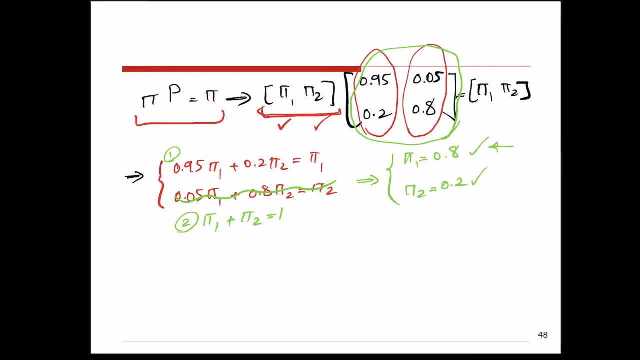 Cola 1 has 80% market share and cola 2 has 20% market share. And if you remember the initial values for the market share for cola 1 and cola 2, Where? so that means the market share for cola 1 has gone from 67% to 80%. 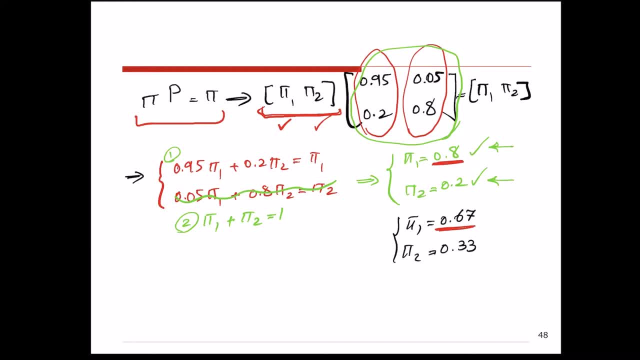 So that's a great progress, but we have to see if this Increase in the market share would bring enough Profit to justify the half a million dollar that we have to pay for that advertisement. so to be able to do so, let's see what is the. 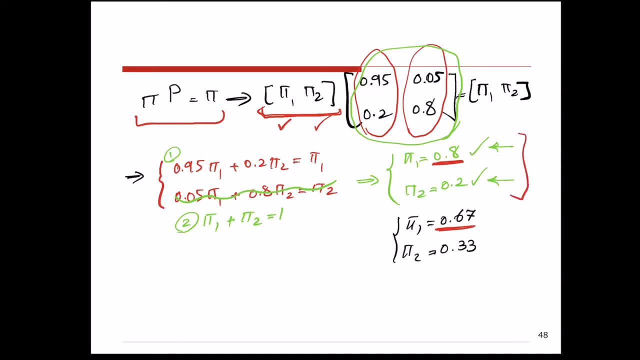 Profit under this scenario, so when the market share has increased. So what is our new profit? if you remember, we have hundred million customers and each one of these customers is going to do, It's going to buy a cola in each week, and we have 52 weeks in a year overall. 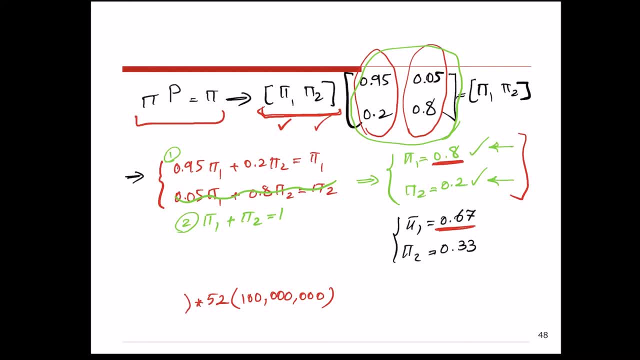 and For each one of these colas we are going to sell it for $2, But at the same time we already have paid $1 as a cost. So we are going to have total $1 as the profit. So this is basically the total profit of this company. 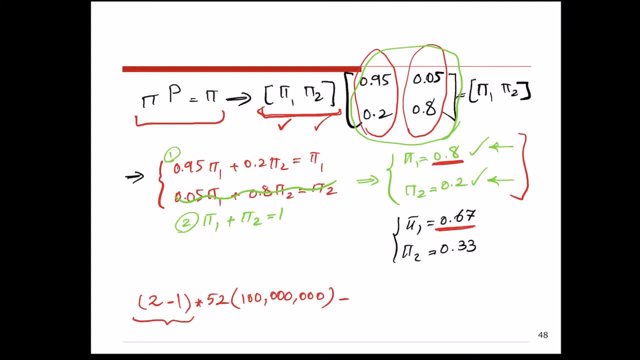 However, we also know that we are. we are going to pay 500 million dollars as the cost of this advertising, So the result is going to be this value. What does that mean? This means that, with this new set up for the transition quality metrics and the 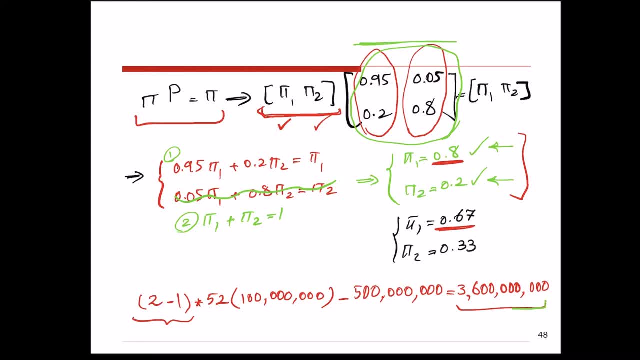 Increase in the market share. it definitely will make sense for us to pay the 500 million dollar for the advertising, Because at the end the profit associated with this advertising Is large. even after we deduct the Money that we have to pay for the advertising, still the profit that is going to stay is large enough. 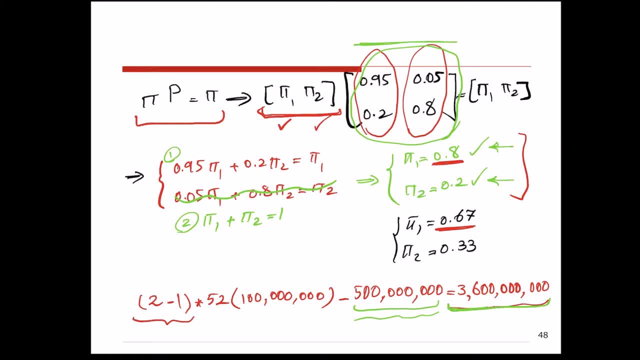 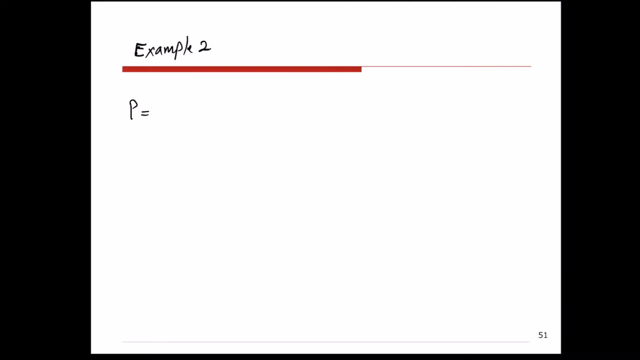 To justify the payment for these ads. So this was just one example as how the Concept of stochastic processes and a steady state properties can be used in a marketing analysis. in the second example, We are going to look at a three by three, one step transition quality matrix. So the transition quality matrix is as below: 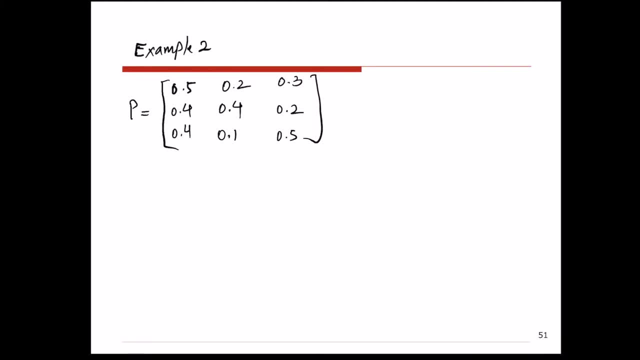 So we want to see what is the, what are the steady state properties in this system? so the first thing, remember we have to check for any stochastic system before we calculate the steady state properties. is that, is this Markov chain and ergodic markov chain or not? because the steady state properties exist only for ergodic markov chain. 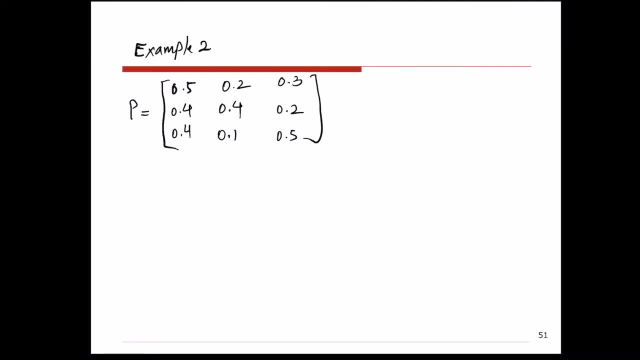 so the three conditions that we have to check for any ergodic markov chain is that if all the states are recurrent, if all of them are Communicating and if all of them are a periodic. So I recommend that you pause the video at this point and check if this mark of change 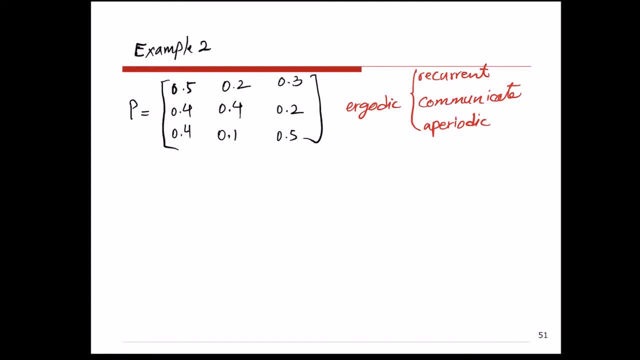 Is an ergodic mark of change. So check these three conditions. So next, to be able to find the steady state properties, We have to solve this famous equations: pi, Vector pi multiplied by one is the transition quality matrix. P equals to vector pi. So that's going to be so, obviously, since in this 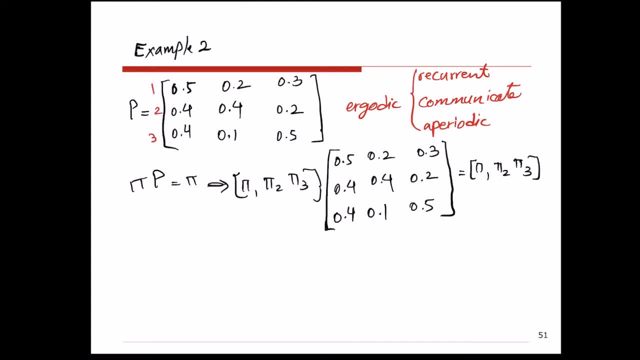 Markov chain. we have three states: state 1, state 2, state 3. our vector pi will have three elements as well: pi 1, pi 2, pi 3. the Stat in the long run, you're in a state 1, you are in a state 2 or we are in a state 3. 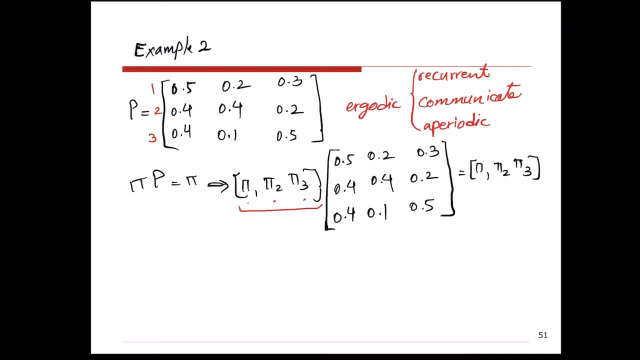 So now let's write down the equations that are coming out of this matrix multiplication. So first we have to multiply vector pi by the first column of the transition matrix P, then we have to multiply vector pi by the second column of the transition quality matrix P, and. 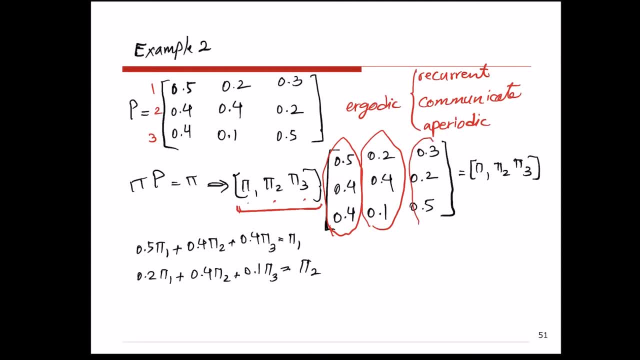 Lastly, we have to multiply vector pi by the third column of the transition party, matrix P, so then these three Equations would come up. So we have three unknowns, pi 1, pi 2, pi 3, and we need three independent equations. so, as I said before, when we put the equations that are coming out of pi, P equals to pi, always, always one of the. 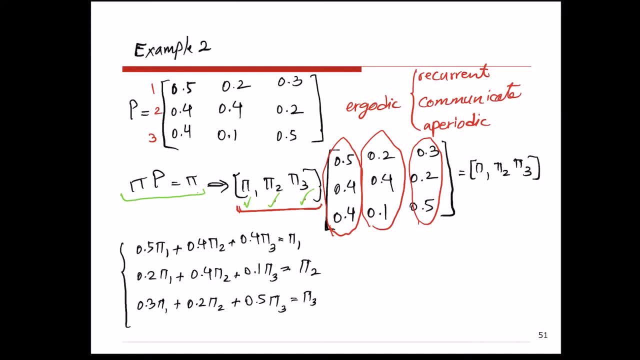 Equations is Dependent to the rest of the equations, so we can drop any one of these equations. so, for example, I'm going to drop equation 1 and I'm going to add that famous equation that holds for all the Mark of chains, so that equation is pi 1 plus pi 2 plus pi 3. 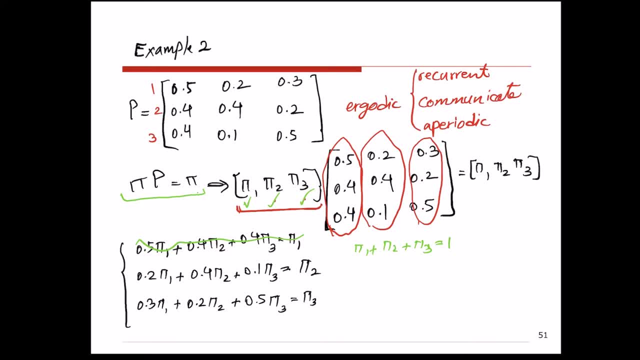 Equals to 1 and as I'm going to write down the other two equations, I'm going to bring all the pies to the left side. So here I'm going to bring the pi 2 to the left side and in this equation I'm going to bring by pi 3 to the left side. So, as a result, these equations are going to be: 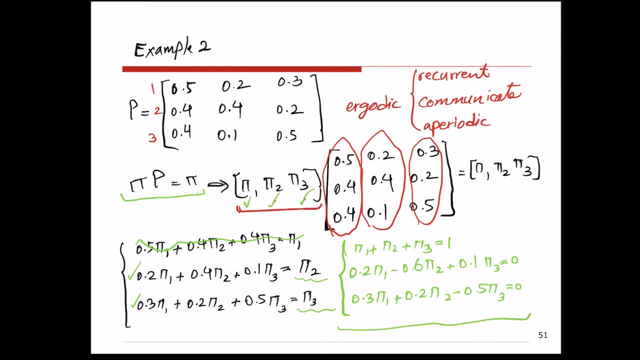 So now we have three Independent equations and three unknowns. we can solve this set of equations to find the answer for pi 1, pi 2, pi 3. To be able to do that, Let's go ahead and write down the matrix representation of these three equations. 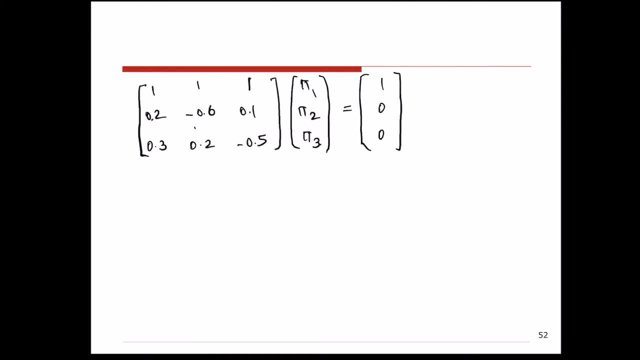 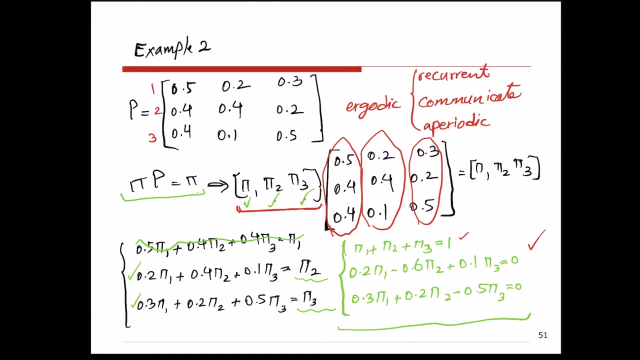 So in this matrix representation of those three equations, As you can see, the first matrix is basically the matrix of coefficients that we saw in previous slide. so, for example, the coefficients of pi 1, pi 2, pi 3 In the first equations are 1 1, 1, and that's what we see in the first row. the coefficients of 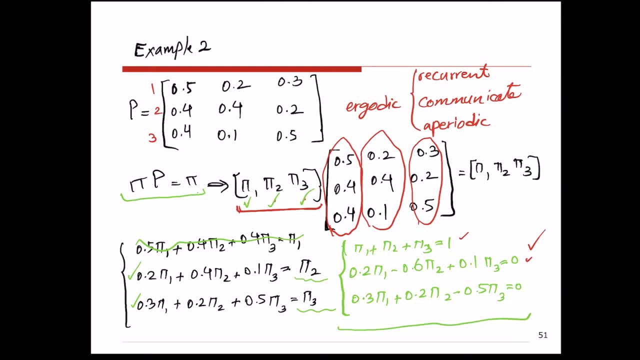 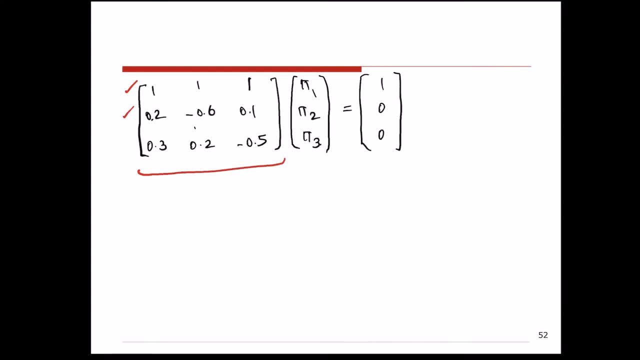 pi 1, pi 2, pi 3 in the second equations- Second equation- are point 2 minus point 6, point 1, and that's what we see in the second row as well, And similarly the numbers that we see in the third row of this matrix are the coefficients of pi 1, pi 2, pi 3 in the third. 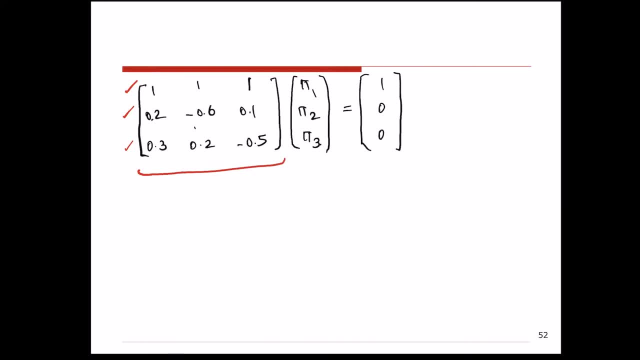 equations multiplied by the Column vector pi and Equation of pi in this matrix. So now that we see this formula, We're going to calculate the sum of pi and the respect that we get here. So what we see on the right side is basically the value that on the, that we see on the right side of those three. 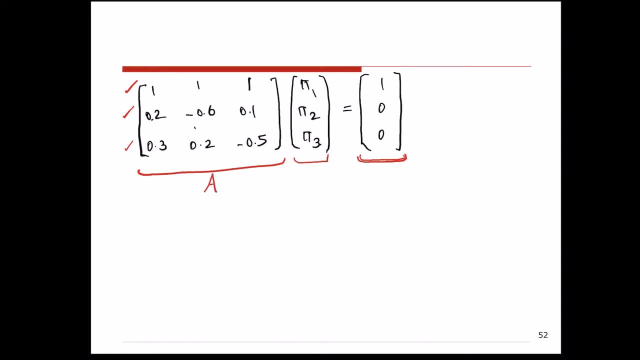 Equations. so the right side value that we see here are 1, 0, 0 and that's exactly what we see here on the right side column vector. So we are going to call this a coefficient matrix. as a to be a multiplied by vector pi equals to b. just pay attention that there are three unknowns: pi 1. 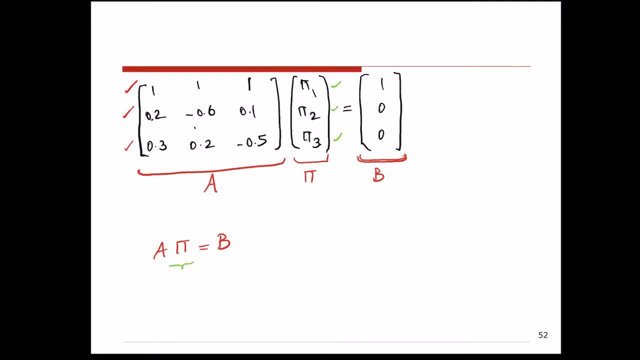 pi 2, pi 3 are in this vector here. so if i want to find a vector pi, what i can do is to multiply both sides of this equation by the inverse of matrix a. so if i multiply both sides of these equations by a inverse, so i will have a inverse multiplied by a. pi equals to a inverse multiplied. 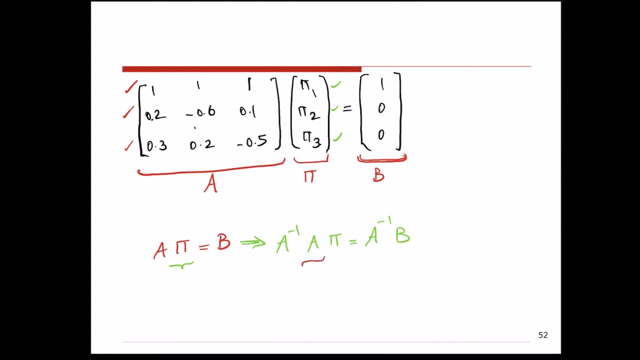 by vector b. as you may remember from the linear algebra, if i multiply any matrix a by its inverse, the result is going to be identity matrix i, and when i multiply identity matrix i by any matrix or vector, the result is going to be the vector or matrix itself. so then, this is: 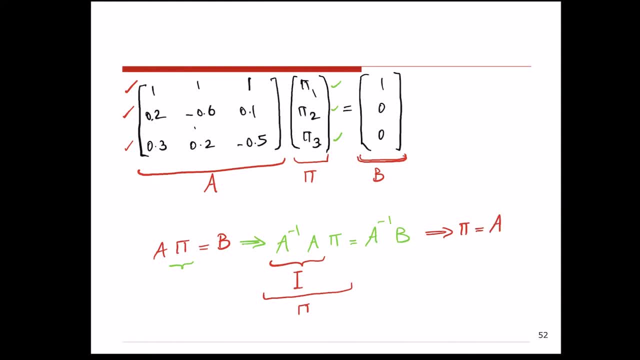 going to be. pi equals to a inverse multiplied by b. so for us to be able to calculate the unknowns in the vector pi, we have to calculate, uh, the coefficient matrix. a then can calculate the inverse of this coefficient matrix and then multiply it by the right hand side, vector b. 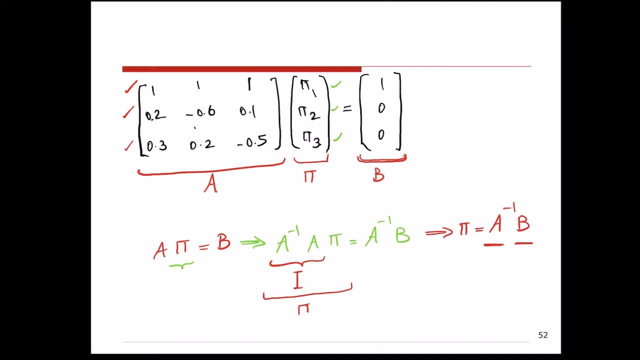 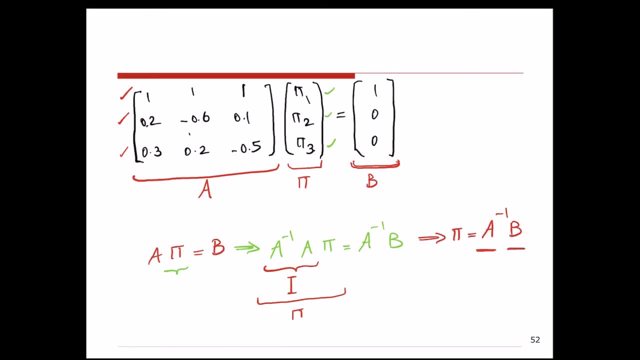 i'll show you next how potentially we can use excel to calculate the inverse of the matrix or the multiplication of the matrices. after the doing the calculations, the value of vector pi is going to be as. so these are the steady state properties associated with state 1, state 2 and state 3. so in 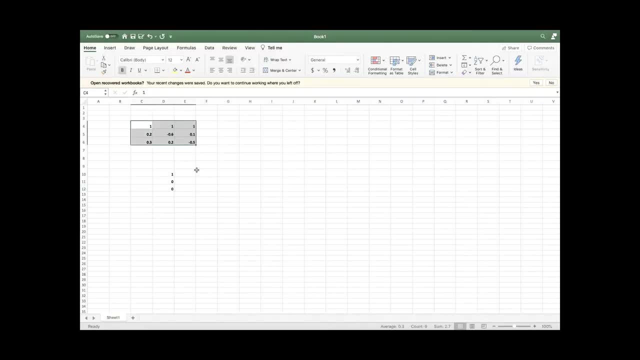 this example: this is the coefficient matrix a and this is the right side, right-hand side, vector P. so the size of this matrix is 3 by 3. the size of the inverse of this matrix is going to be 3 by 3 as well. so first I highlight a 3 by 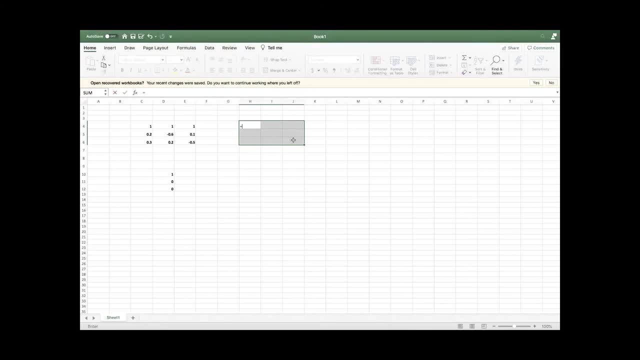 3 area, and then I put equal and then M- inverse, matrix, inverse, and then I pick the array or the matrix that needs to be inverse, I click the frances and then I have to press SHIFT CTRL dan ENTER, and this is going to be the inverse of the matrix. it's very, very. 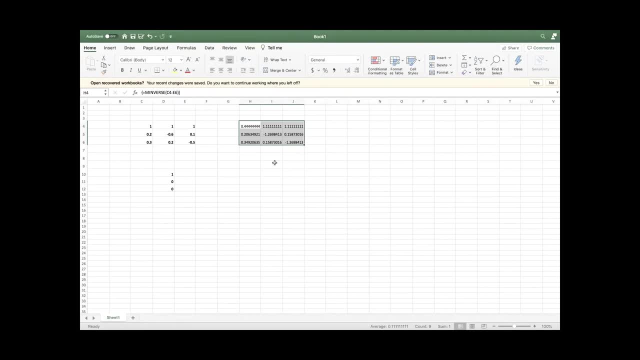 important for you guys to press SHIFT CTRL and ENTER, and not just the ENTER for me. And then we see the inverse of the matrix here. So now this is the inverse of the matrix A, And we know that we have to multiply the inverse of matrix A by vector B. 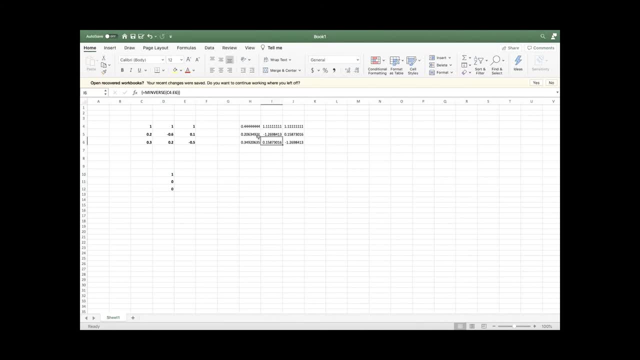 So the inverse of the matrix A is a 3 by 3 matrix. The vector B is a 3 by 1 matrix. The result is going to be a 3 by 1 matrix as well. So first highlight the cells that represent the dimension of the results. 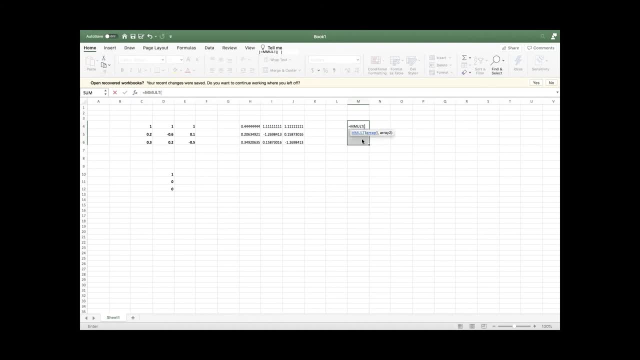 Then equal M, M mult. matrix multiplications is basically what we have to use as a function. And then we pick the first matrix, that's A inverse, and then comma, And then we pick the second matrix, that's vector B. 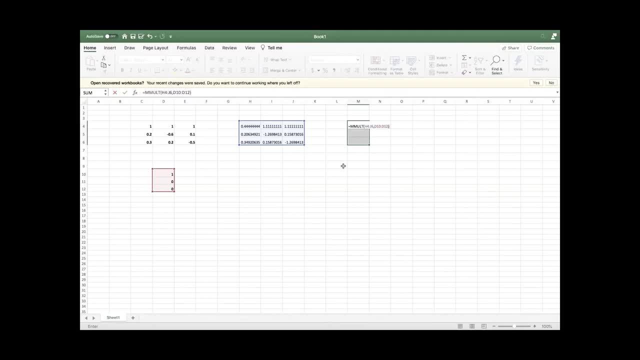 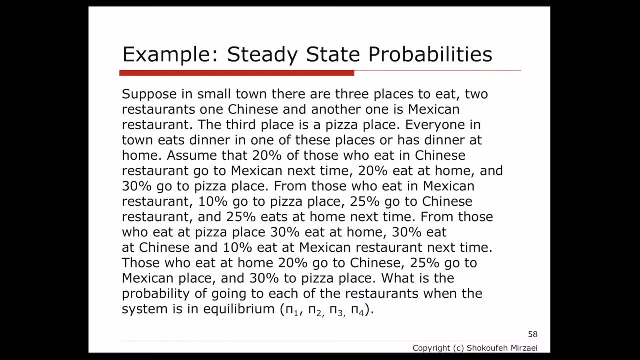 And then close parenthesis And again shift, control, Enter. So this is going to be the results. The last example that we have are related to the restaurants in a city. So in a specific city there is a Chinese restaurant, Mexican restaurant and a pizza place. 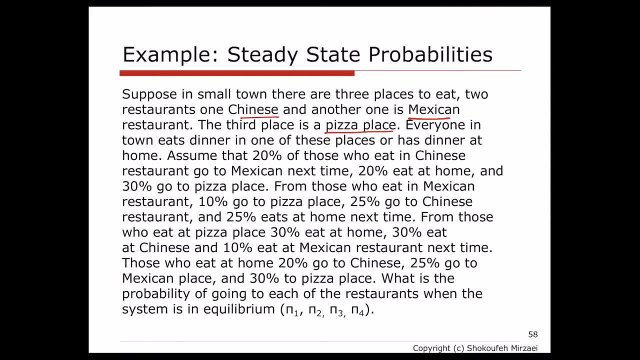 So people have the option to eat in any one of these restaurants or eat at home. So assume that 20% of people who eat in a Chinese restaurant right now will go to a Mexican restaurant For their next meal. 20% of them will eat at home and 30% of them go to a pizza place. 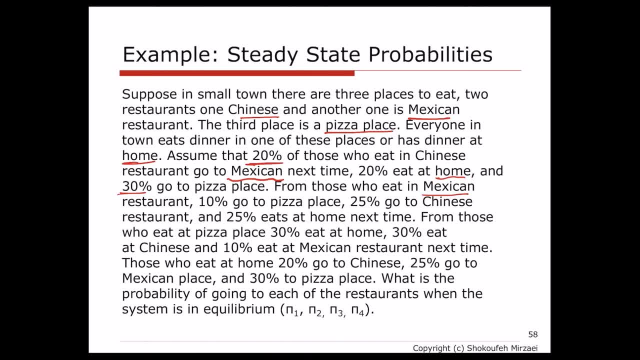 From those who eat in a Mexican restaurant right now, 10% of them will go to a pizza place for their next meal, 25% will go to Chinese restaurant and 25% will eat at home. And from those who eat at the pizza place right now, 30% of them will eat at home for their next meal. 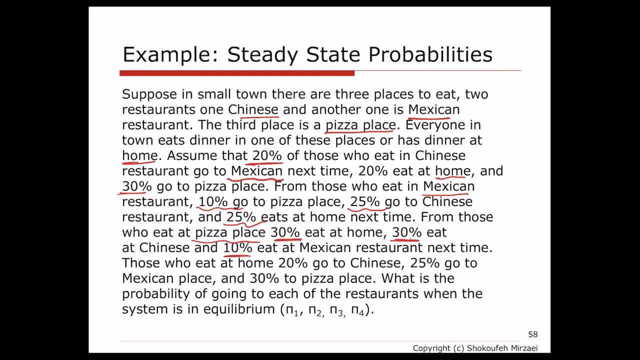 30% of them will go to Chinese restaurant restaurant and 10 percent of them will go to a mexican restaurant. and lastly, for all of those people who eat at home, 25- 20 percent of them will go to a chinese restaurant in their next meal. 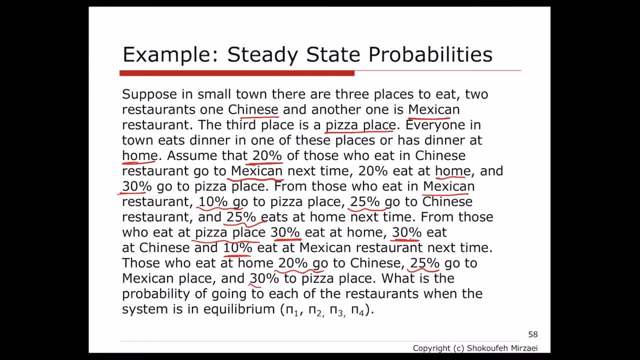 25 percent will go to mexican and 30 percent will go to a pizza place. so we want to calculate the probability of going to each one of these restaurants when the system is in equilibrium. so that means in the long run, in the city state in the equilibrium if we stop this city and pick 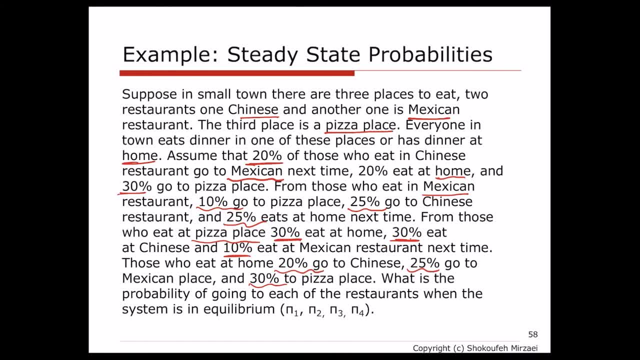 any person in this city, what is the probability that they are eating in a at home, or at the chinese restaurant, or at the mexican restaurant, or as at the pizza place? so those are basically city state behavior of this system. so basically, what we want to do is to find the values of 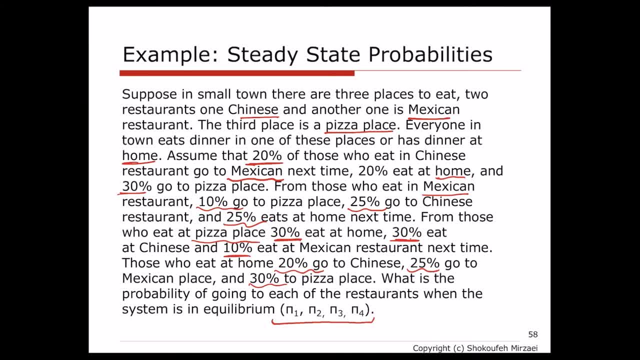 vector pi you. So let's assume pi 1 shows the probability that the person is eating at home. pi 2 shows the probability that the person is eating at the chinese, pi 3 shows the probability that the person is eating at the mexican restaurant and finally, pi 4 shows the probability that the person is eating at the pizza place. so we want to. 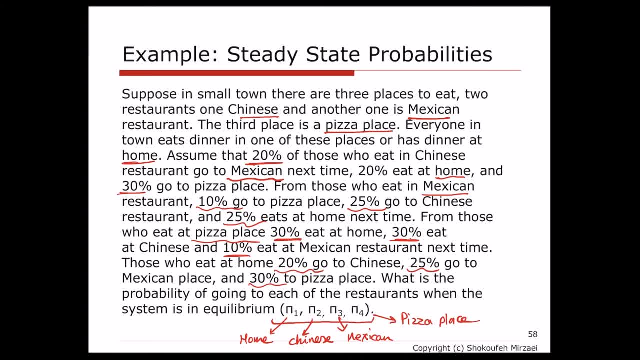 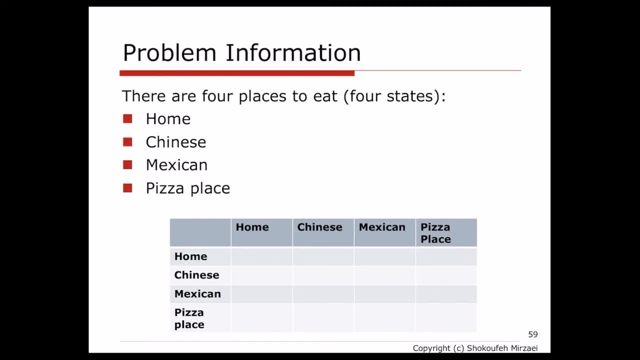 go ahead and find the values of vector pi for this stochastic system. so now let's go ahead and put this transition probabilistic part metrics together. so obviously, the state of the system, which is the place in which people eat or the type of food that people eat, has four values. 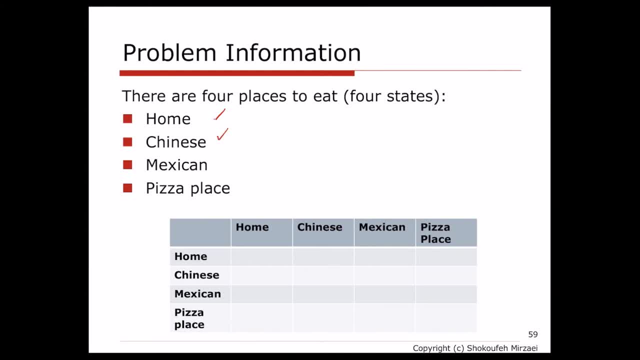 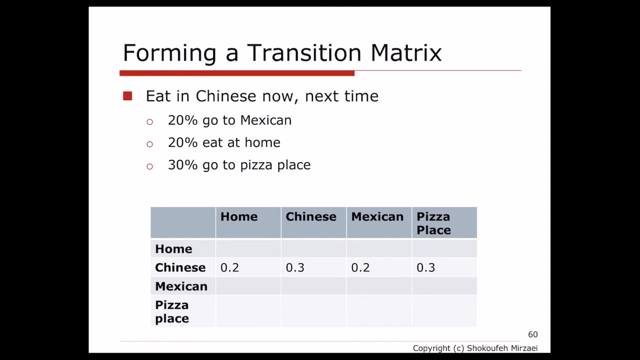 value. one means the chance of eating at home, eating to chinese, eating at mexican and eating as a at the piece of place. so the one is the transition property metrics. p will be a 4x4 metrics. so so from the problem statement that we know if a person is eating at the chinese restaurant, 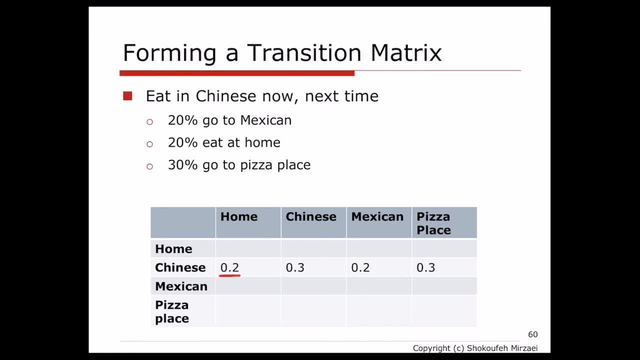 restaurant right now, there is 20% chance that for the next meal the person eats at home, 20% chance that the person is eating at the Mexican restaurant and 30% chance that the person is eating at the pizza place. And one minus the sum of this value is the probability. 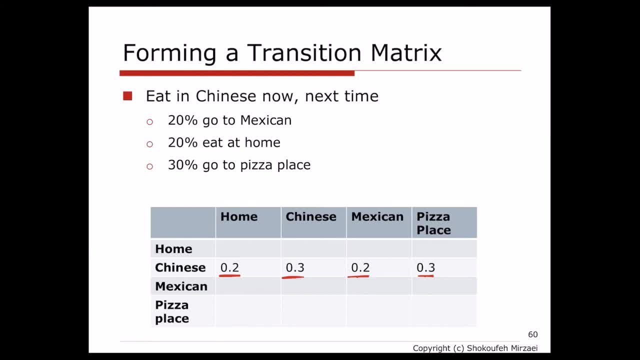 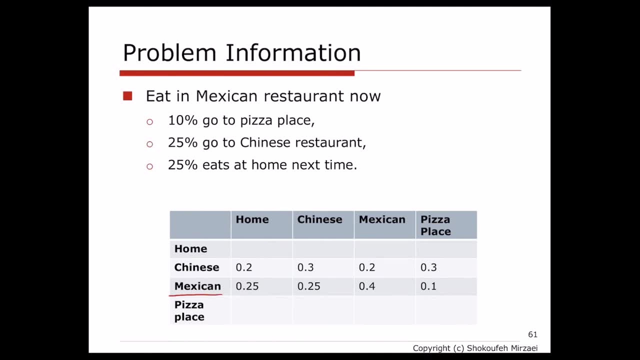 that the person continues eating at the Chinese restaurant. If a person is eating at the Mexican restaurant right now, there is 10% chance that the person is going to eat at the pizza place in the next meal. there is 25% chance that the person is going to eat at the Chinese place for the next. 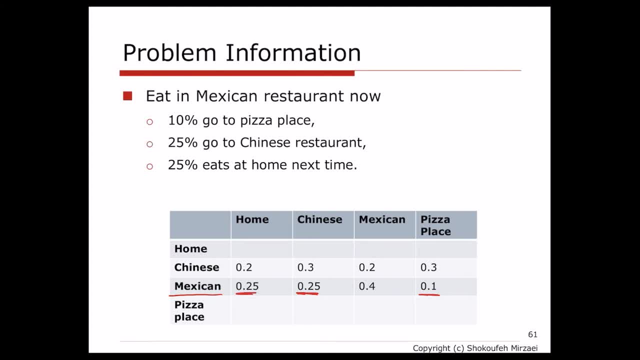 meal, there is 25% chance that the person is going to eat at home and one minus the sum of these probabilities is going to show that 40% chance. there is 40% chance that the person is going to continue eating at the Mexican restaurant. And if the person is eating at the pizza place right now, 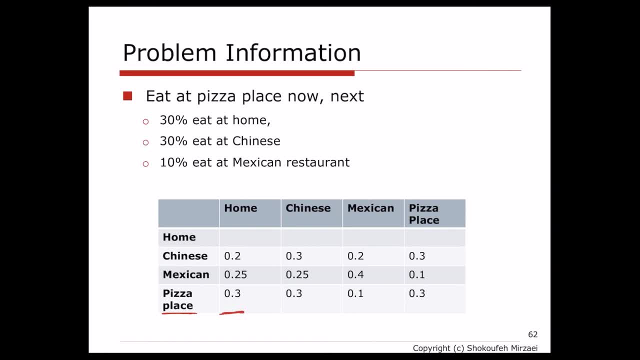 there is 30% chance that the person is going to eat at home for the next meal, 30% chance that the person is going to eat at the Chinese place And if the person is eating at the pizza place restaurant, and 10% chance that the person is going to eat at the Mexican. 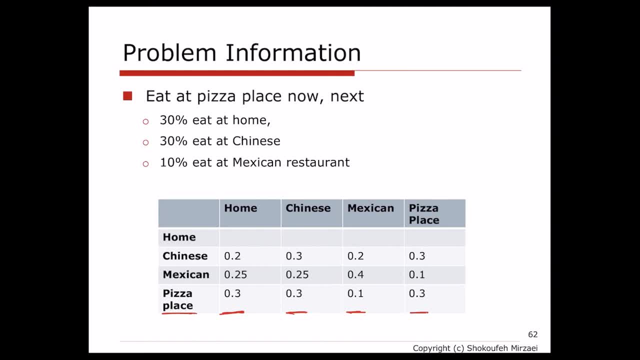 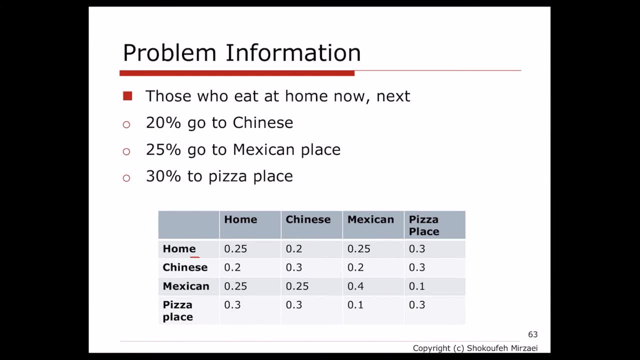 restaurant and one minus the sum of these values, it shows that there is also 30% chance that the person is going to continue eating at the pizza place and, lastly, if the person is eating at home right now, there is 20% chance that the 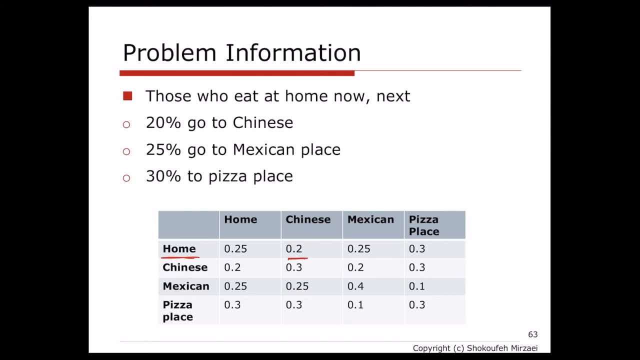 person is going to eat at the Chinese restaurant for the next meal. 25% chance of eating at the at the Mexican place and 30% chance of eating at the pizza place and one minus the sum of these values shows 25% chance for continuing. 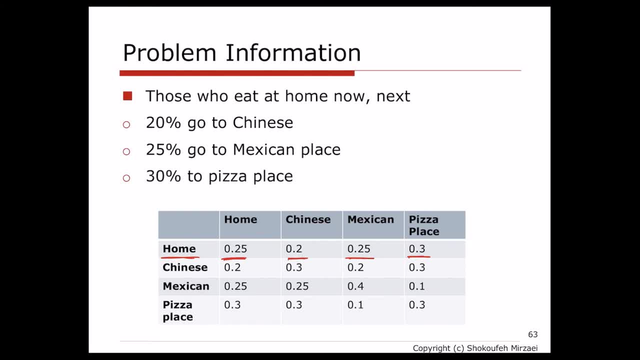 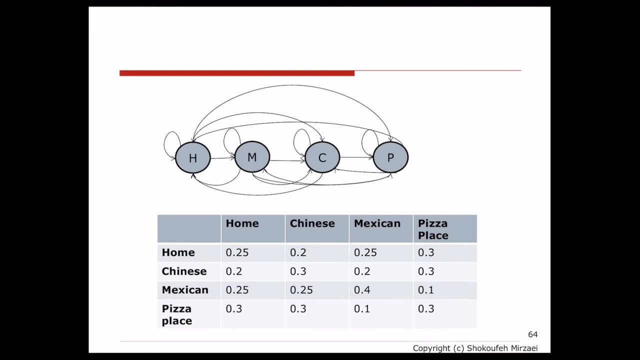 eating at home for the next meal. so this is the one-step transition probability matrix for this problem that we extracted from problem state. so now, before we go ahead and calculate the steady state probabilities, we have to find out if this Markov chain is ergodic. and remember the three conditions for a. 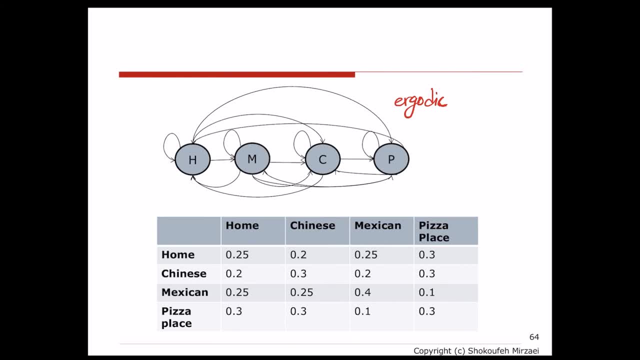 Markov chain to be ergodic is that all the states are recurrent, they come, communicate and they are a periodic at this one. I want to ask you guys to pause the video and check if these three conditions hold in this Markov chain. so next we are going to go ahead and find the steady state transition problems for. 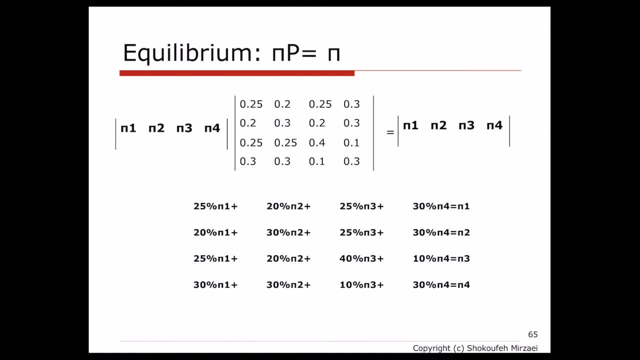 this stochastic system. to do so we have to first put our famous equations of PI- P equals to PI- together, as I said, since there are four possible states in the system. the vector pi- the steady state, probabilities- has four elements: pi 1,. 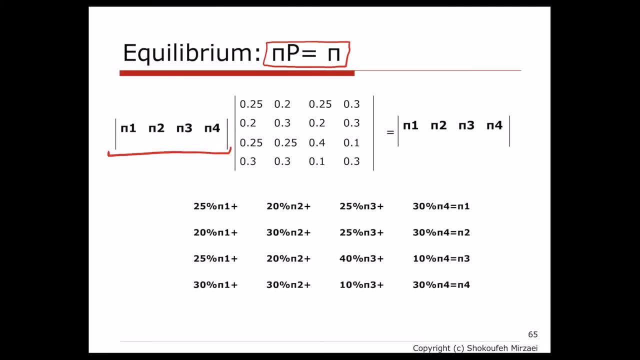 pi 2, pi 3, pi 4.. So this vector is going to be multiplied by one step transition probability matrix P, which is going to be equal to vector pi. So now we have to multiply vector pi by the first column of matrix P, and that's going to be the first equation. Then we multiply vector pi. 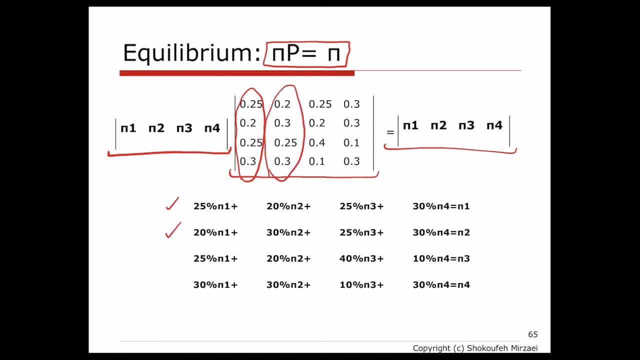 by the second column of vector P- that's going to be the second equation- then by the third column and then by the fourth column, and those are going to be the third and fourth equations. So we have four unknowns. those are the elements of vector pi, pi 1 to pi 4, and we need four. 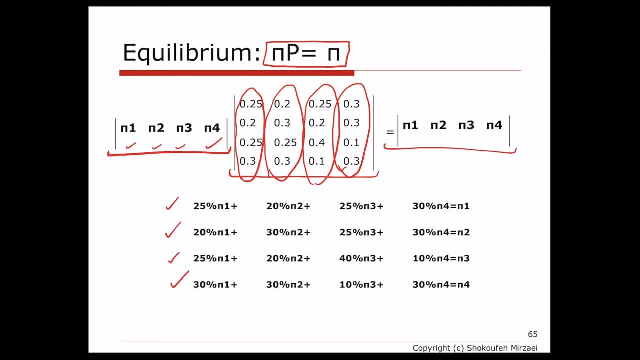 independent equations so that we can solve the set of equations that we have and find the values of those four unknowns. But, as I have said several times, when we put together the equations that are coming out of pi, P equals to pi, always, always one of. 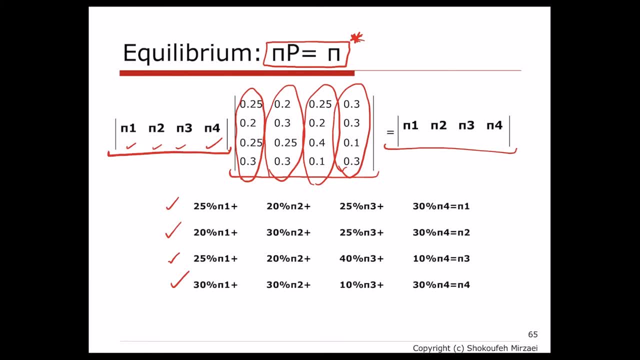 the equations is dependent to the rest. So we can drop any one of these equations, it doesn't matter. And for example, here I'm going to drop the first equation and I'm going to add the famous equation that we have for the 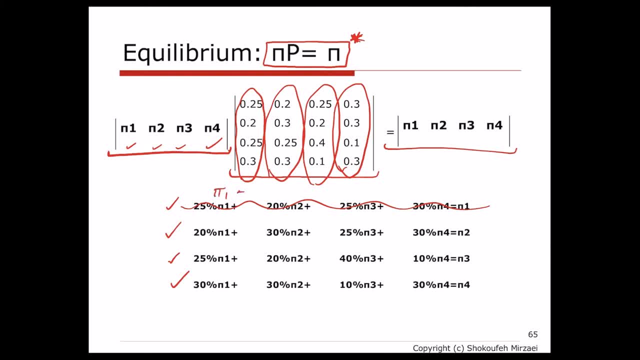 states of a system, which is pi 1 plus pi 2 plus pi 3 plus pi 4, equals to 1.. As I have said before, why this equation holds? Because in the long run, the system is finally at one of these states. The system is either at state 1 or state 2, or state 3 or state 4.. 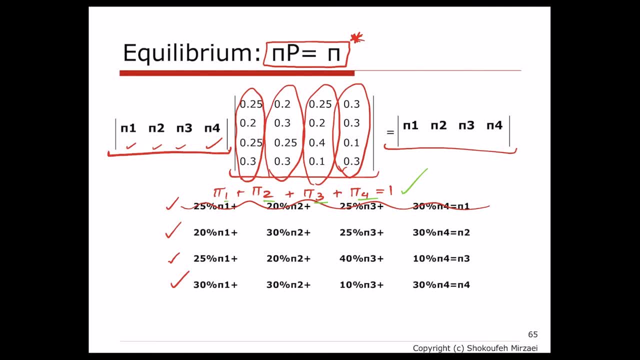 So, as a result, the sum of these probabilities end up to be equal to 1.. So now I have four equations, and these equations are independent from each other, So I can solve them to find the values of the set of properties. So to do so, for the other three equations, I'm going to take the pi's to the left side of. 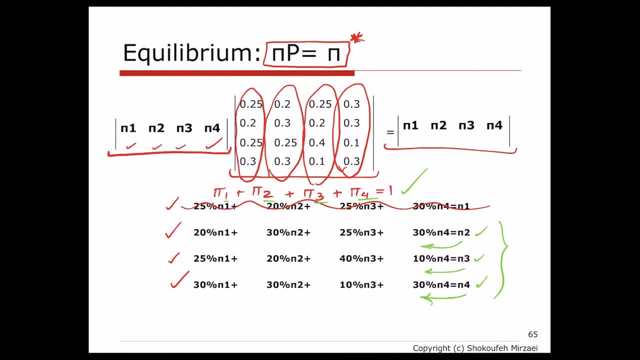 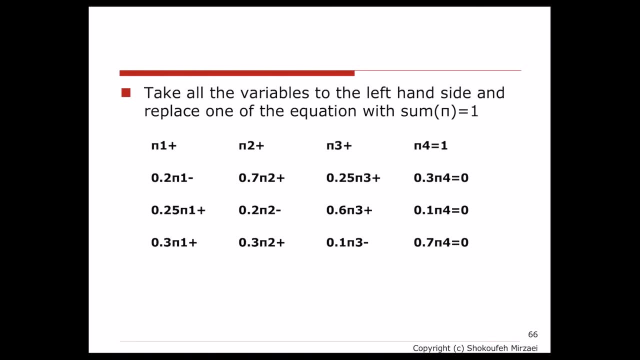 the equation And, and if I do that, the final results are, as we can see here. now we have four independent equations For unknowns. we can solve them to find the values of the set of properties. So first, remember, based on the formula that we said was that vector pi equals to A inverse. 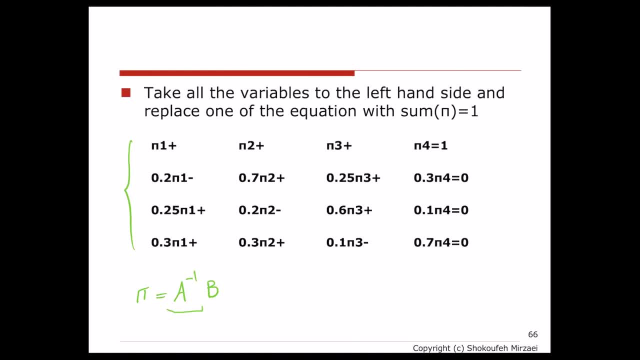 multiplied by vector B, What is A inverse? So matrix A is the matrix of coefficients in this set of equations and matrix and vector B is the vector of the right-hand side of the equation. Let's try to find that vector B here, maybe A to the dû vector of A. 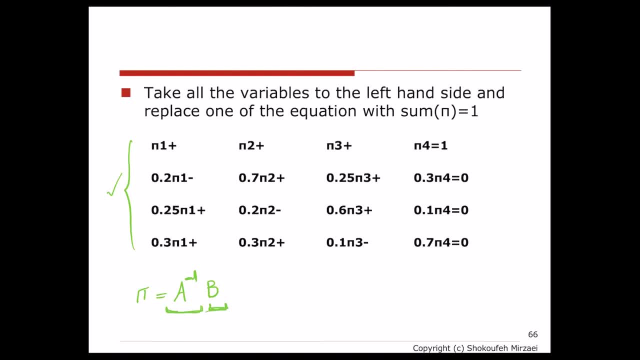 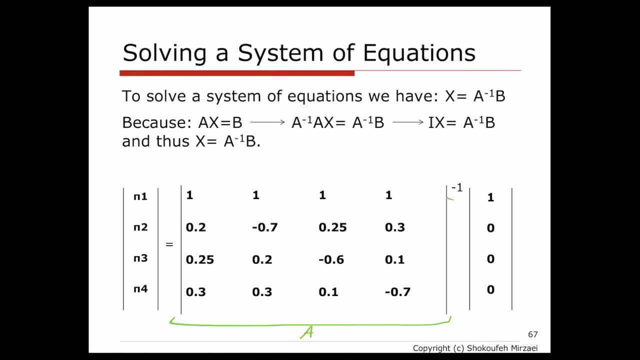 And if we find the matrix in here and multiply it with the vector A, all either side of the equation will be the population. So we can check. the matrix got from A. this is also A inverse of A. So I am going to let me just videoga camps with you. 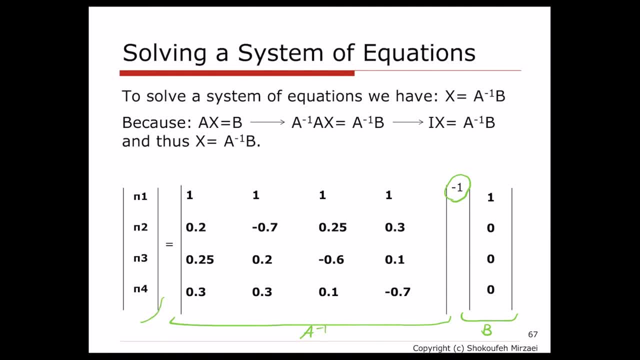 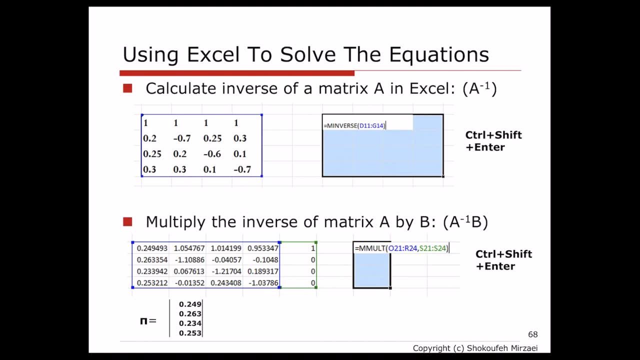 Let's give it a vote. So this matrix, This matrix must be the university of England. give us the values of the vector pi and, as we showed before, we can use excel to find the inverse of matrix a and um and also then multiply this inverse by the right hand side vector p, so to: 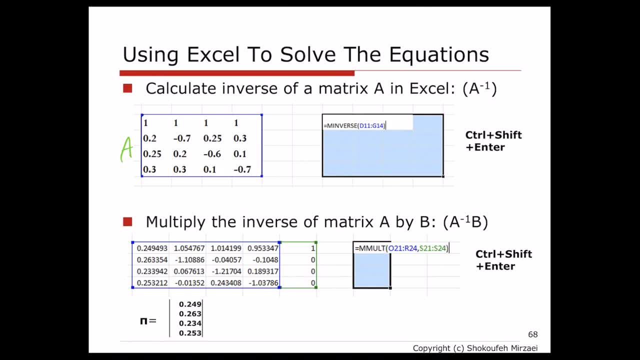 find the inverse, we have to. we can potentially use the function m inverse, that's matrix inverse, that exists in excel. and to be able to multiply the inverse of matrix a by the right side, right hand side, vector b, we can use the function m molt, which is related to matrix multiplications. 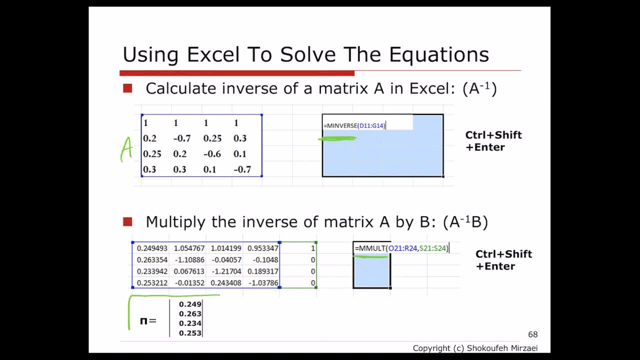 if we do that, the final values for the steady state properties is what we have shown here. so these are the values for pi 1, pi 2, pi 3 and pi 4.. so these values are going to help us to see. in this example. we have some values for pi 1, pi 2, pi 3 and pi 4. so these values are going to help us to see in the 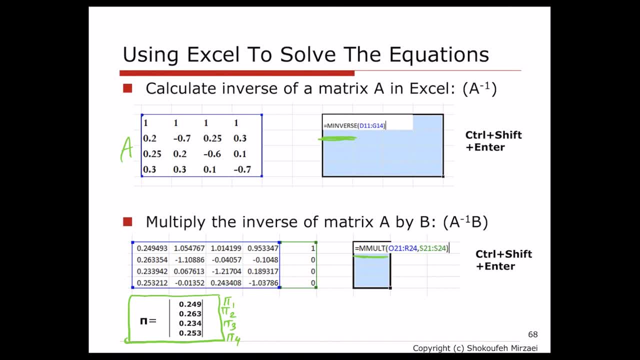 the long run when the system reaches and city-state. if we stop the system and we pick any customer from this city, what is the chance that they are eating at home? what is the chance that they are eating at the Chinese restaurant? what is the chance that they are eating at the Mexican restaurant and what is the